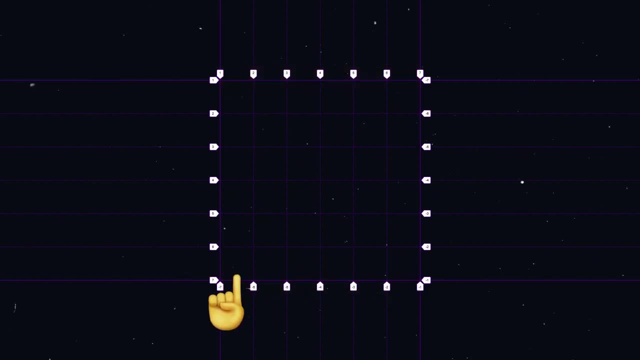 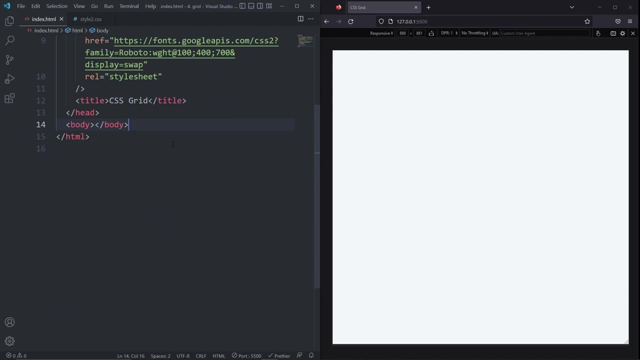 Our grid is made up of cells. Each square is a cell And, finally, our grid is also made up of tracks. These are the rows and these are the columns. Creating a grid starts in the HTML. We need a container and some items inside of it. 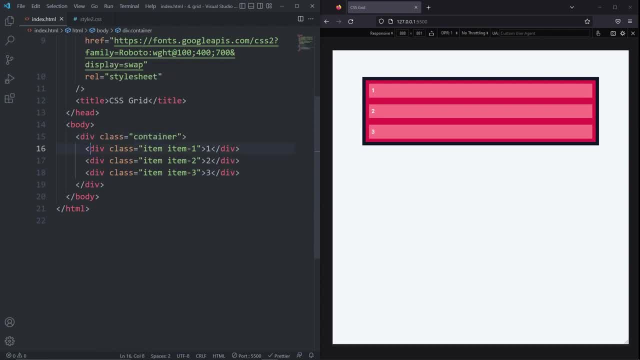 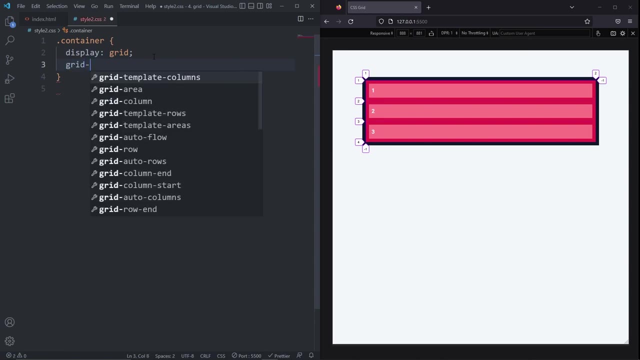 The container is a div with the class of container and the items are divs with the class of item: item1,, 2, and 3.. In our CSS, we give the container the display of grid. We see nothing happened, but this is because we need to tell grid how many rows and columns we want defined. 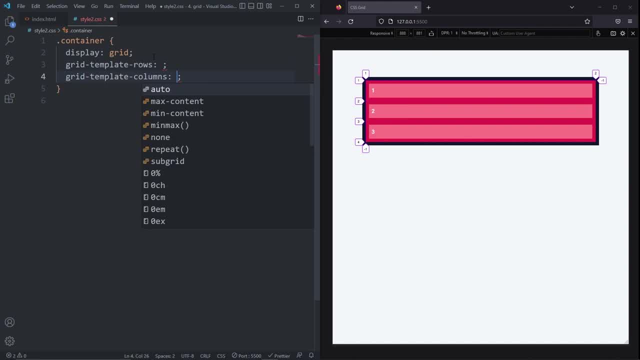 To define rows and columns. we use the GridTemplateRows and GridTemplateColumns properties. They work by defining a track for each value that you pass it. If I give 100 pixels to the columns now, I have one column of 100 pixels. 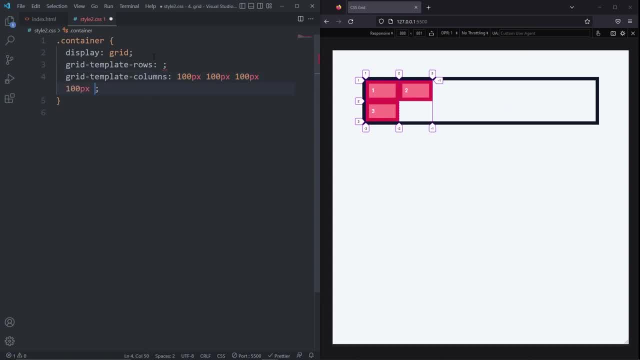 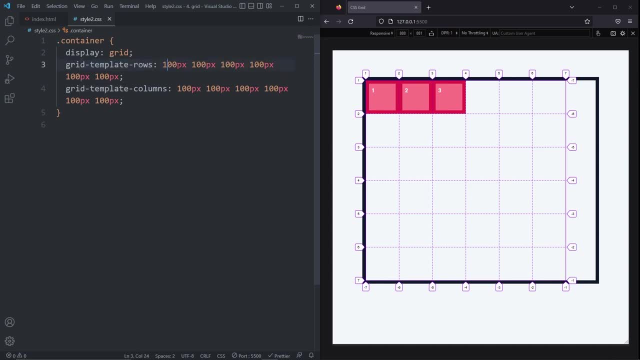 If I add a second value of 100 pixels- now I have two columns of 100 pixels, and so on- I'll copy the values from my GridTemplateColumns and paste them in the GridTemplateRows. Now I have a grid with 6 rows and 6 columns, and all of the cells have the same size. 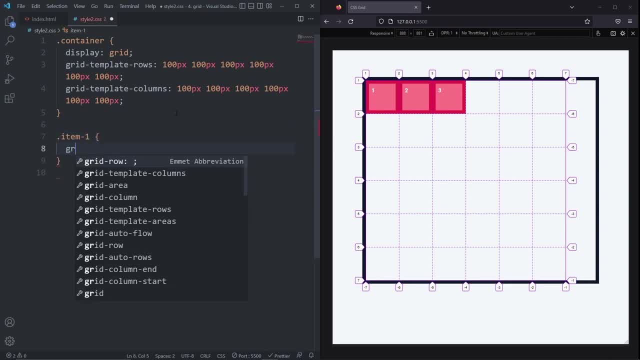 If I want to position an item, I can select it and give it the GridRowStart, GridRowEnd, GridColumnStart, GridColumnEnd properties. Inside of each will go some line numbers. Let's say I want item 1 to look like this: 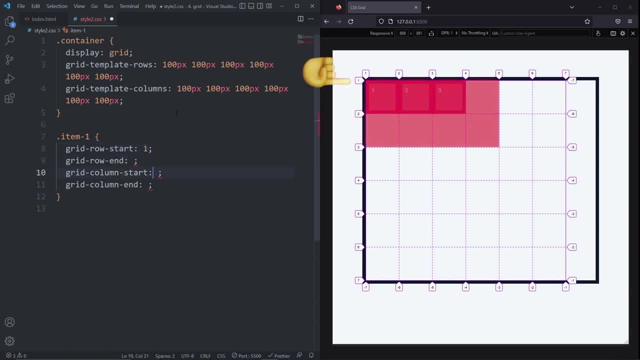 Then that means item 1 starts on line 1 of both the rows and the columns. We also see that item 1 ends on the third line of the rows and ends on the fifth line of the columns. The other two items were pushed because we aren't explicitly defining their position. 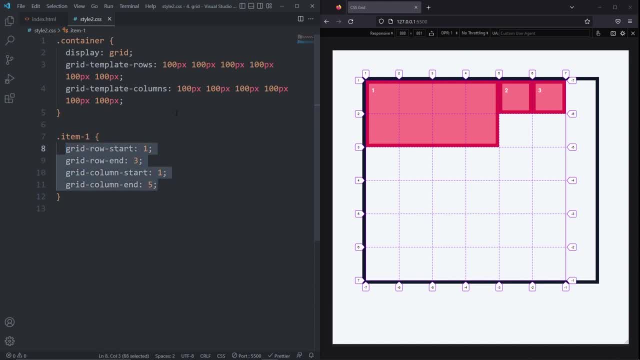 Writing these four properties each time you want to position something is a bit much. You can instead use these two shorthand properties, GridRow and GridColumn. Like the other properties, these also take inline numbers as values. The first value is the starting line. 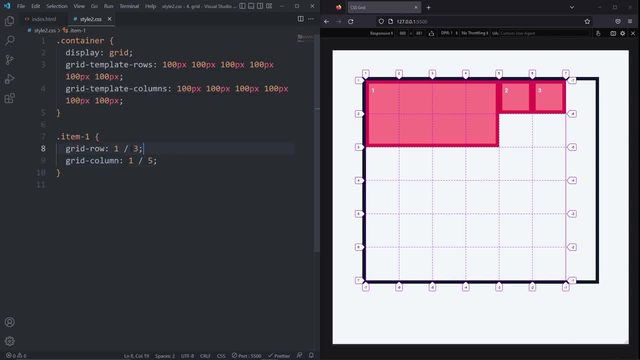 the second is the ending line and they need to be separated by a slash. I want my second item to span 2 rows and columns. I could give it a GridRow of 1 and 3, and a GridColumn of 5 and 7,. 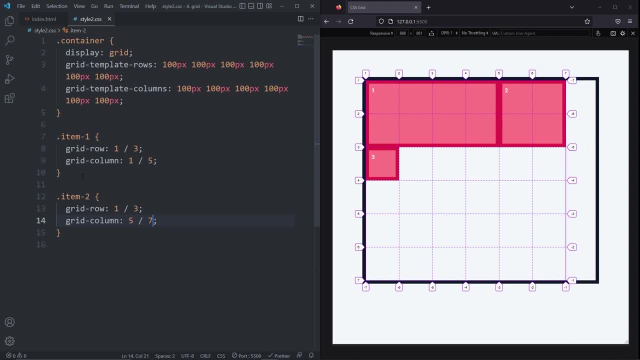 and this works amazingly. but an easier way to achieve this is with the span keyword. Instead of the values that I currently have, I can just use the span keyword with the number of cells that I want to span. basically, the span keyword is saying: from wherever you currently are. 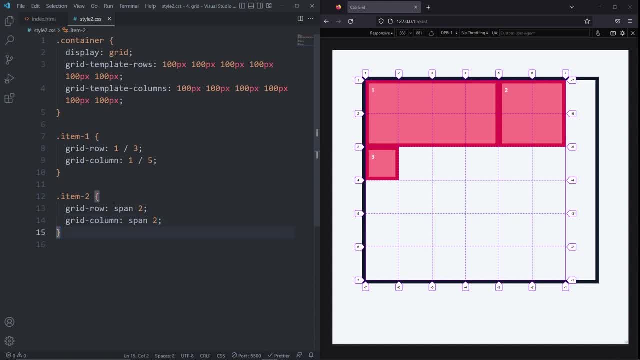 span yourself this number of times. This is easy to read and is also why a lot of people love the span keyword, but the main downfall of using this is it doesn't allow you to explicitly define your starting and ending position and, as a consequence, our item will be pushed away. 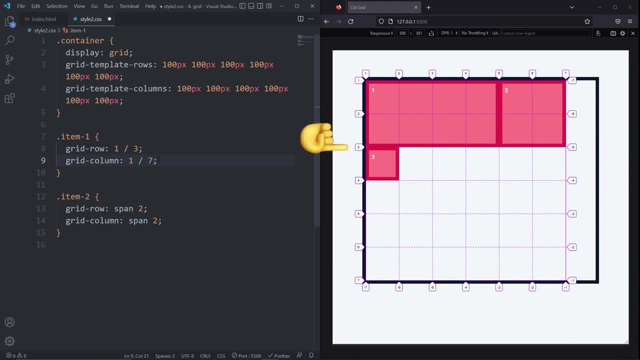 if I increase the size of a nearby item, like item 1.. If you don't care about anchoring an item into a specific position, then the span keyword is okay to use. Using GridRow and GridColumn is good, but there is an even faster property. 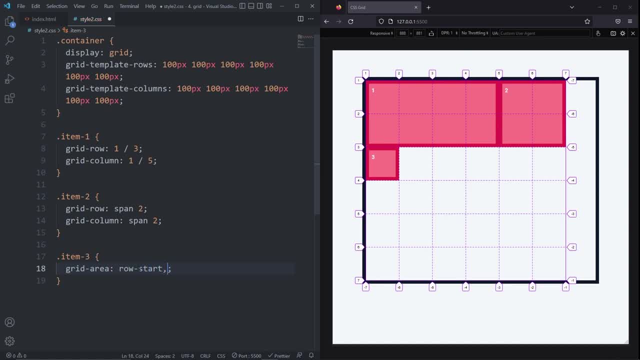 GridArea takes 4 values: the first is the starting line on the rows, the second is the starting line on the columns, the third is the ending line on the rows and the fourth is the ending line on the columns. If I want item 3 to fill out the rest of the available space, 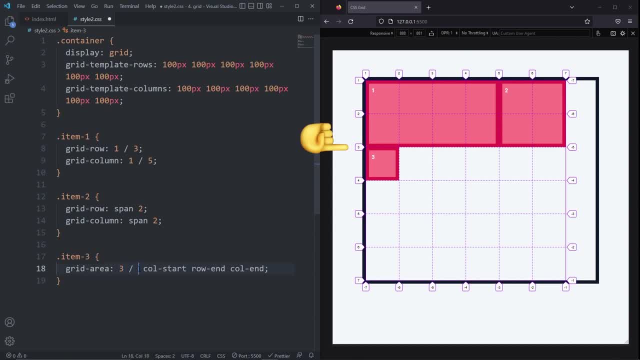 I can give it the GridArea with the starting row of 3, the ending column of 1, the ending row of 7, and the ending column of 7.. I can also use the negative numbers that we see on our grid. 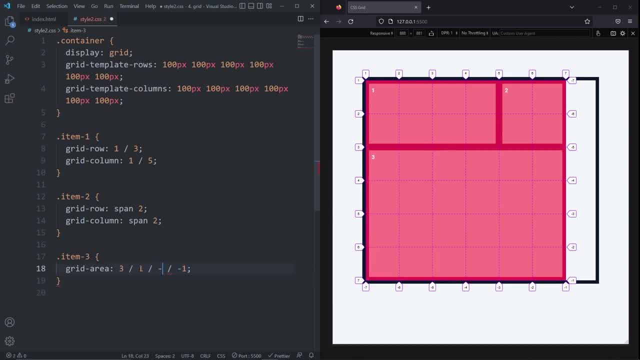 So instead of 7 and 7, I could say minus 1 and minus 1, and this will work the same. This one property does the job of 6 properties, so personally, that's the one that I always use. Before CSS Grid. layering an item on top of another was painful. 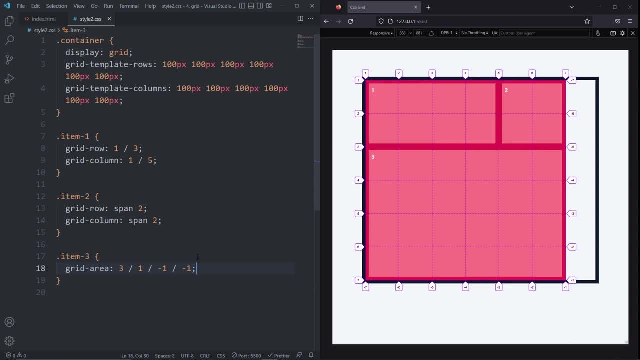 You had to use an absolute positioning and then try to position the item using the top, right, bottom and left properties. But with CSS Grid you just position your item where you want it to be and, if that happens to be, on top of another item. 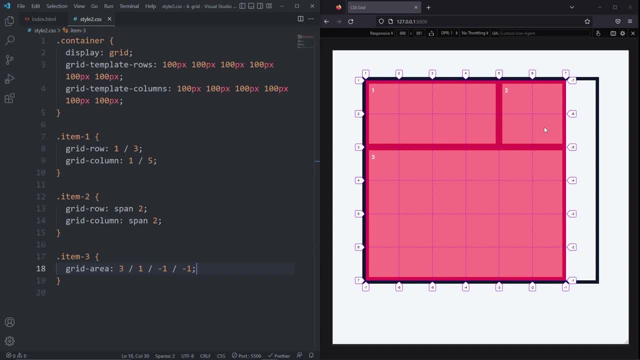 then that creates layering Super easy. I want item 2 to be right here, touching both the item 1 and item 3.. To do this, I'll remove the grid row and grid column and use the grid area instead. 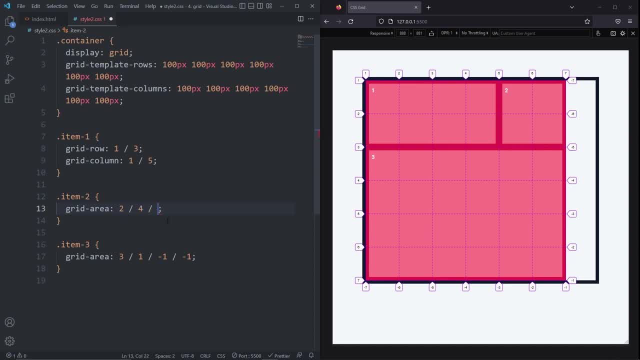 The row starts at 2, the column starts at 4, the row ends at 4, and the column ends at 6.. Our item needs to be on top. All we have to do is give it a z-index of 1,. 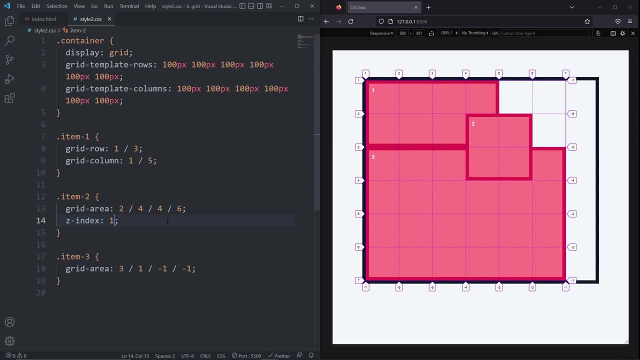 and now item 2 is layered on top of both item 1 and item 3.. Now we see our items are filling out all of the available space, except maybe for the top right corner. I'll make item 1 span all of the columns just to fill everything up. 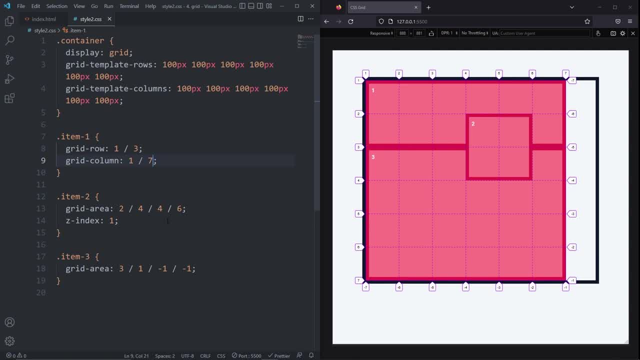 So, now that all the cells are occupied, what would happen if I added another item in our HTML Despite not having any room left? our grid added a new row for item 4.. When items are added outside of the explicitly defined grid, this is referred to as an implicit grid. 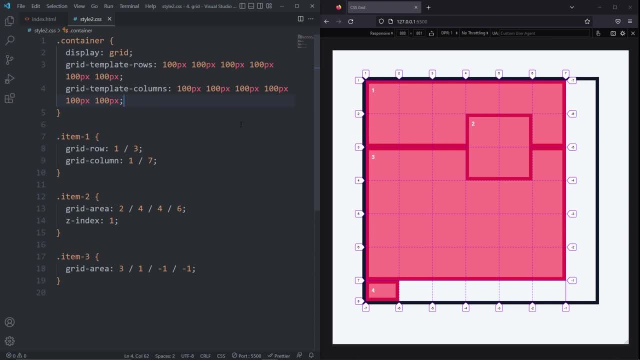 Notice how item 4 is smaller than the others. That's because the implicit grid doesn't inherit the values that we set in the gridTemplateRows and gridTemplateColumns properties, But what we can do is add the gridAutoRows property on our container. 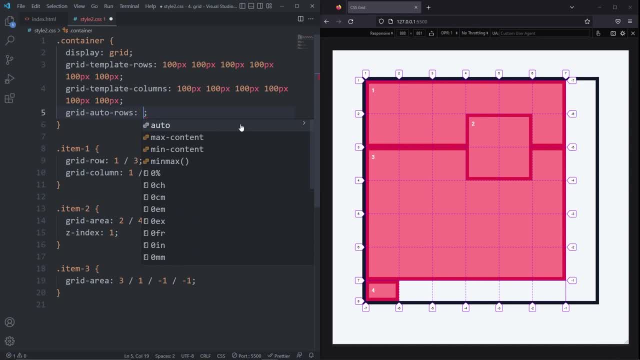 What this does is sets the size of the rows on any implicit grid that gets created. I set it to 100px. Now our implicit grid has a row of 100px By default. our implicit grid added a row, But we can change this with the gridAutoFlow property and set it to column. 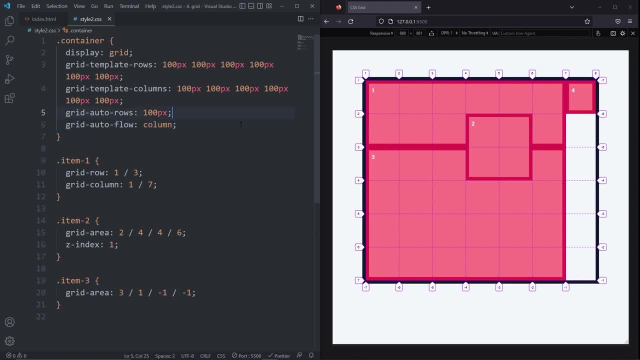 Now, any implicit grid that gets created will be created as a column instead, With the columns being the new default for our implicit grids. we can use gridAutoColumns to define the size of those columns and set it to 100px. Now let's reset our grid by commenting on it. 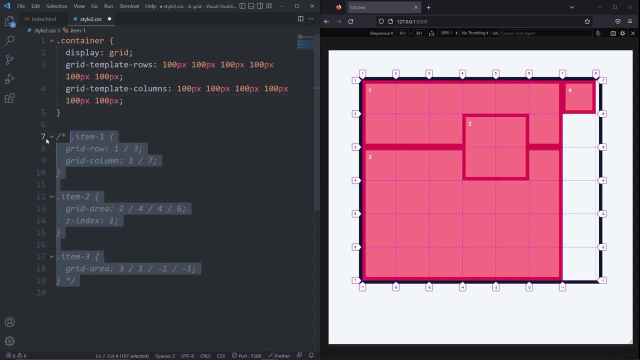 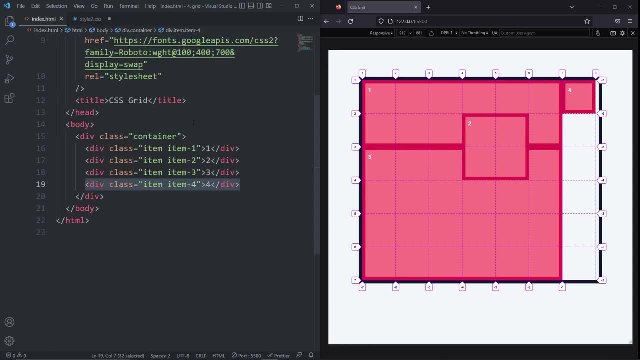 The gridTemplateRows and gridTemplateColumns properties are the same. Inside the gridTemplateRows and columns can go more than just pixel units. You can use ems, rems, percentages, etc. But there is one called the fractional unit that you should know about. 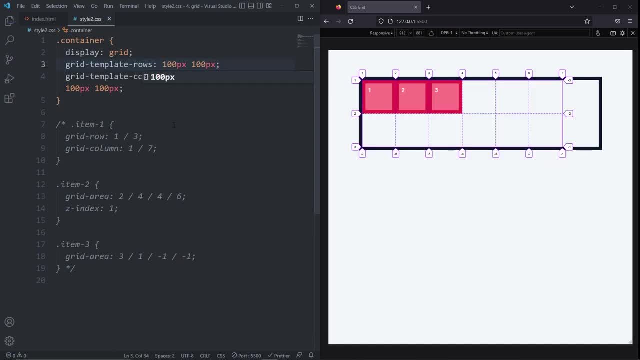 I'm going to give the rows two values of 100px and I'll give the columns three values of 1fr. The fr unit represents a fractional value of the available space, and now we've got three columns, each one filling out the available space. 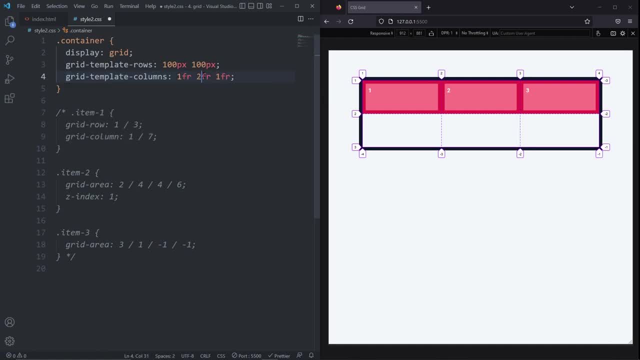 If I set the second fr to 2 or 3,, we see the column occupying more of the available space. You can also mix the fr units with other units without any issues. so, for example, I can make the first value be 100px. 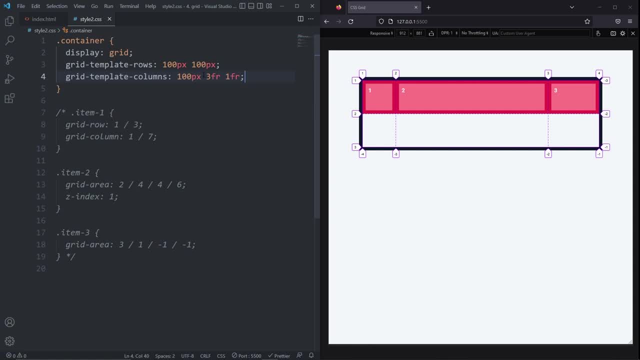 In general, you can mix and match values without any problems. When I resize the page, some of the items get way too thin. To set a minimum width, we can use the minmax function inside our gridTemplateColumns. I'll use the minmax function on the second column. 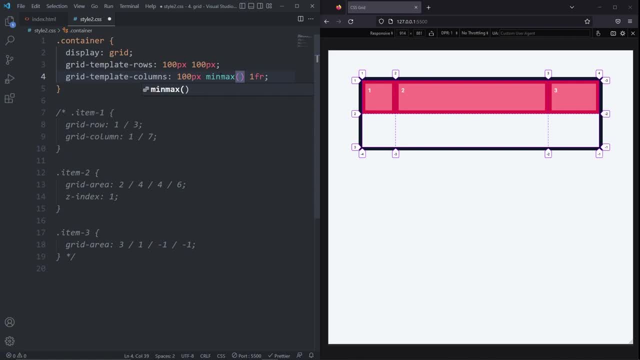 It takes two arguments. the first is the minimum size and the second is the maximum size. I'll set the minimum size to 100px and the maximum size to 3fr. Now our item will stop shrinking whenever it hits 100px. 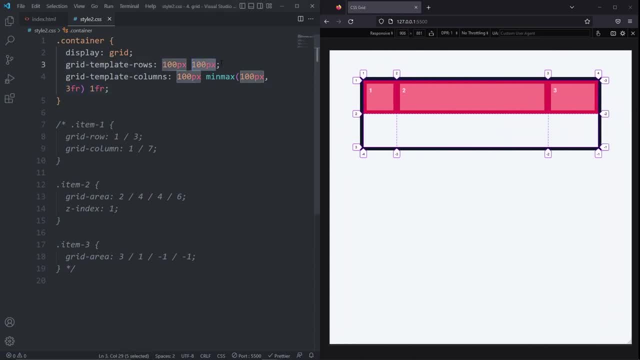 Another useful function is the repeat notation. I'll use this one on my gridTemplateRows. The way the repeat notation works is by taking two arguments. The first argument is the number of times you want to repeat a value, and the second argument is the value you want to have repeated. 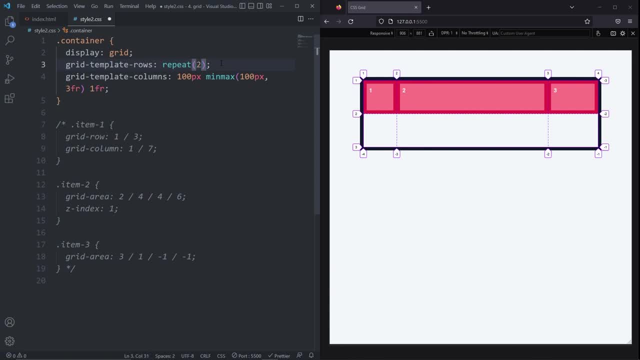 We had two values of 100px, so I'll set the first argument to 2, and the second argument to 100px. Now the rows are just like they were before: two rows of 100px. but now at least we aren't repeating ourselves. 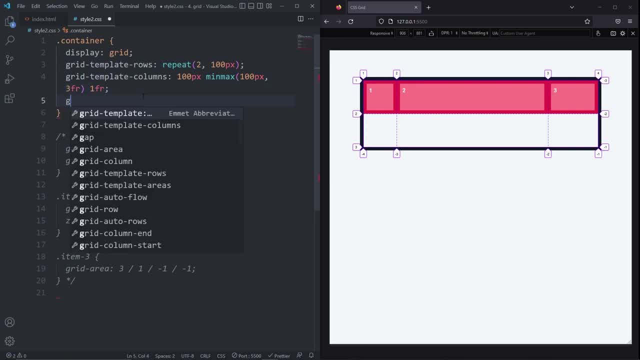 We can also add gaps to our grid with the gridGap property. If you assign it one value, then it will add gaps equally to both the rows and the columns. If you assign it two values, the first is the gaps on the rows and the second value is the gaps on the columns. 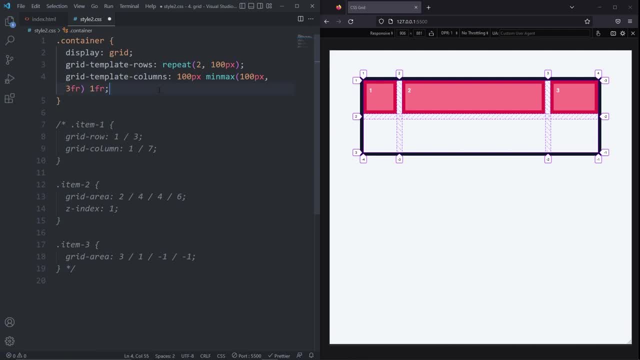 I'm going to replace the values in my gridTemplateRows for 100px, 300px and 100px. I'll also replace the values inside my gridTemplateColumns for 1fr and 3fr. I'm going to show you another way of positioning items in your grid. 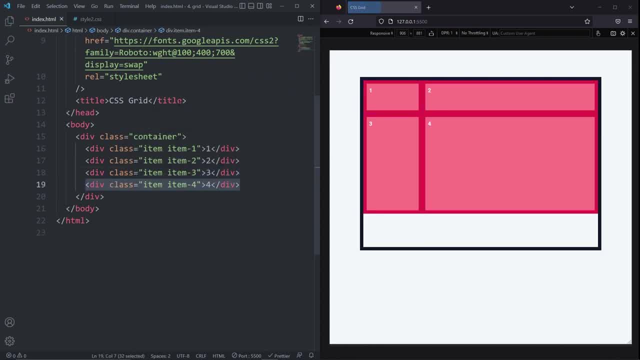 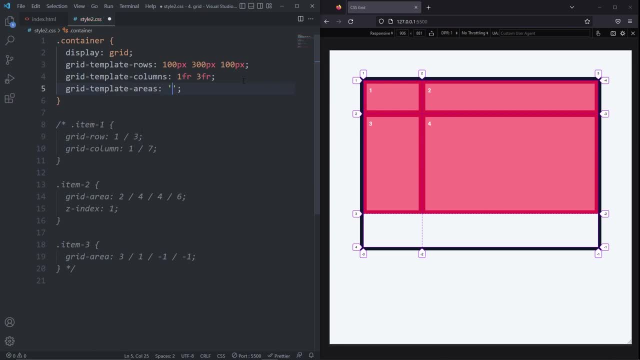 that doesn't require keeping track of the line numbers In my container. I'll add the gridTemplateAreas property As a value. I'll give it three sets of single quotes stacked on top of one another, with a semicolumn after the last set of single quotes. 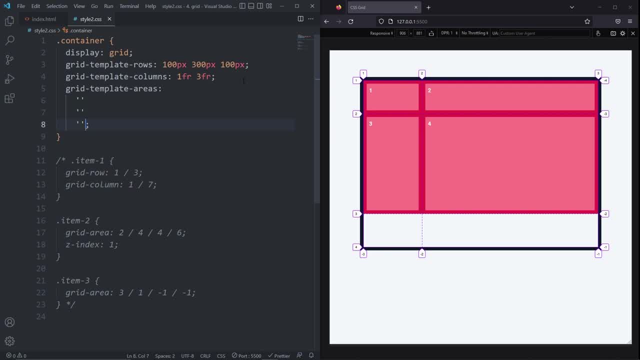 Looking at my gridTemplateRows, I see I defined three rows. and looking at my gridTemplateColumns, I see I defined two columns. We have three rows and two columns. Well, inside the first set of single quotes, I'll say header and header. 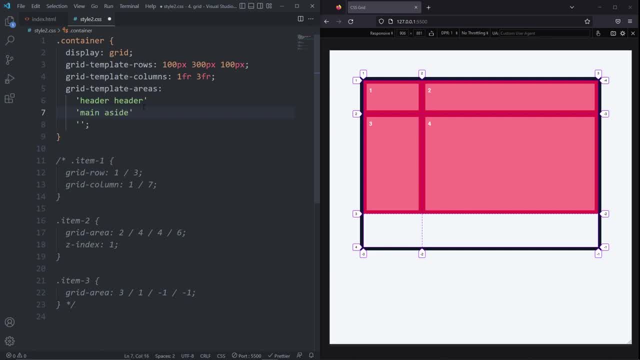 Inside the second set of single quotes I'll say main and aside. Inside the third set of single quotes, I'll say footer and footer. The reason I added three sets of single quotes is because I know my grid only has three rows. and the reason I added two values inside of each of the single quotes. 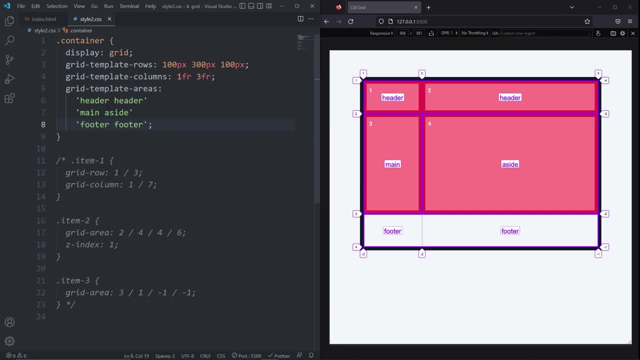 is because I know my grid only has two columns. Each set of single quotes represents a row and each value inside of them represents a column. Looking at my grid, we see the developer tools added the names we set inside the gridTemplateAreas in the appropriate position. 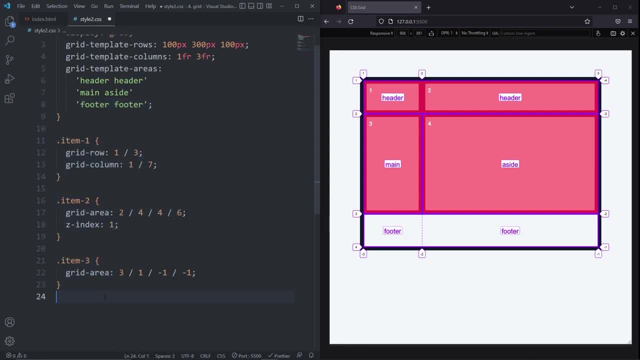 Now all I have to do is give each item the gridArea property and assign them the section I want them to occupy. I want item1 to be the header, I want item2 to be the main. I want item3 to be the aside. 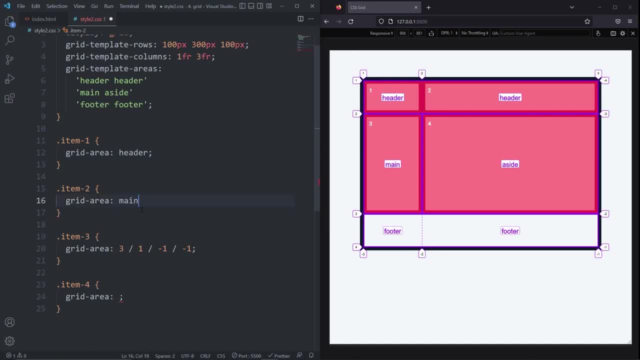 and I want item4 to be the footer. Now we see each item is occupying the section we assigned them to. By the way, this was just an example. I don't think I'd have one grid for all four sections in a real website. 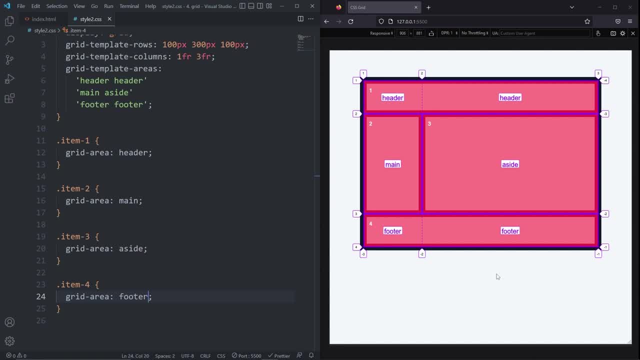 I'd probably have multiple different grids across my page for the various sections and components. Also, this way of positioning things is fun, but it makes layering items more difficult. It can be done, though, it's just more difficult. We're almost done. 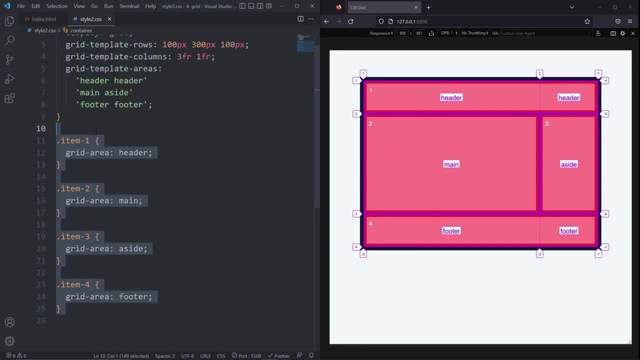 I'll reset my grid by commenting out pretty much everything and set a repeat of 4- 100px on the rows and a repeat of 4- 1fr. on the columns. Our items are currently stretching both on the row axis and the column axis. 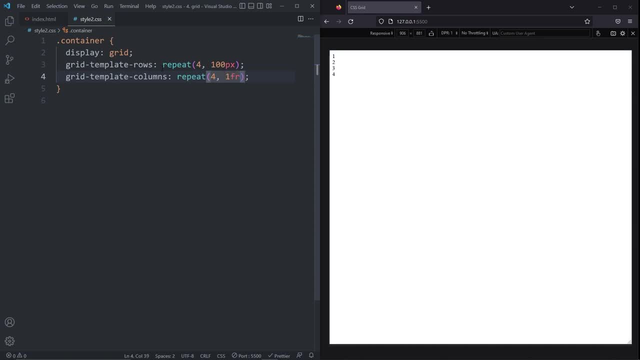 and this is because on our container there's two properties we don't currently have but that in the background, have a default of stretch: The justifyItems and the alignItems properties. both have a default value of stretch. I can change them to either start, end, baseline or center. 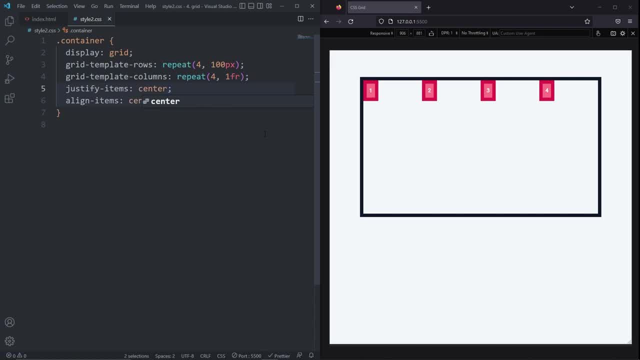 justifyItems align items on the row axis. so if I change justifyItems to anything else, like start, we see our items are at the start of the row axis but still in the center of the column axis If I change alignItems to anything else. 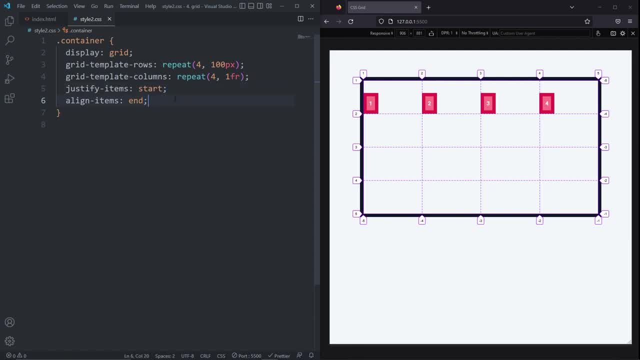 like end. now our items are still at the start of the row axis, but are now at the end of the column axis. These properties are affecting all of the items, but if we wanted to align items individually, we can use the justifySelf and the alignSelf properties. 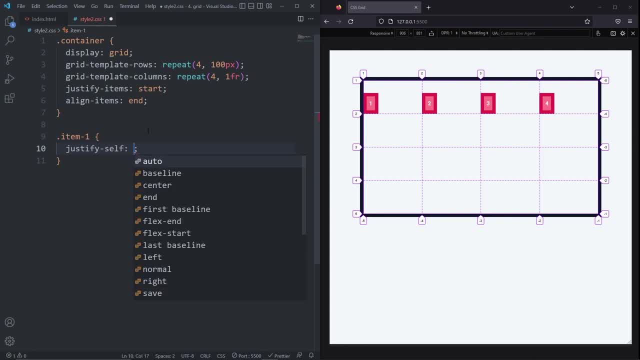 on the items themselves. So, for example, if I wanted to overwrite the row alignment of item 1, I could use the justifySelf and set it to anything else like center. and if I wanted to also overwrite the column alignment, I would use the alignSelf property. 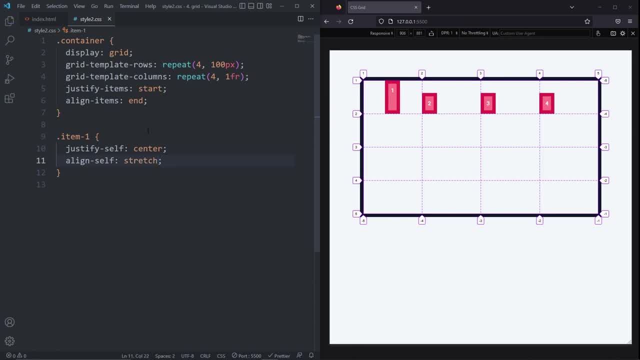 maybe this one- I'll set it to stretch- justifyItems and alignItems were to align our items inside our grid, but we can also align the grid itself along the container. So, for example, I'll clean things up by removing everything except display of grid. 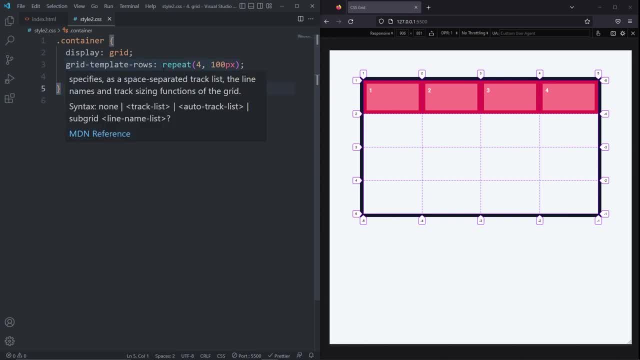 gridTemplateRows and gridTemplateColumns. I'll also add a height to the container of 600 pixels. I'll say that we have 2 rows instead of 4, and also 2 columns instead of 4.. I'll also replace the 1fr with 100 pixels. 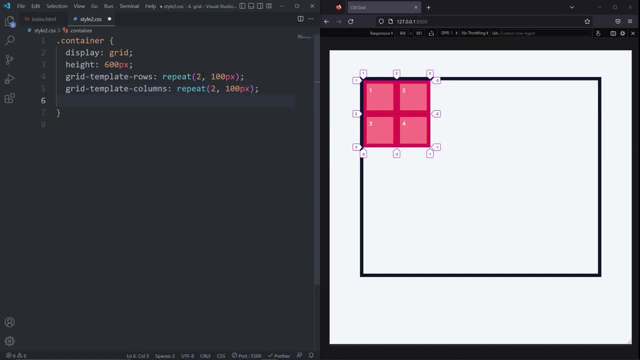 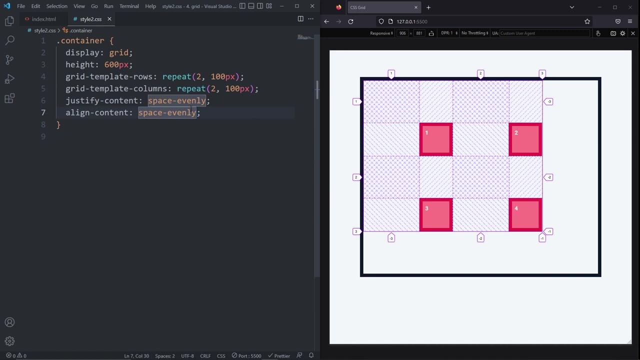 Now we have a smaller grid in comparison to the container. We can align the grid with justifyContent and alignContent. They both take the same values- start, end, center, baseline, space between space around and space. evenly, justifyContent aligns the grid along the row axis. 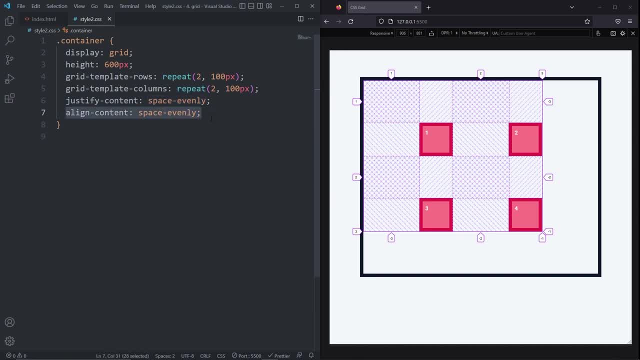 and alignContent aligns the grid along the column axis. The last thing I want to show you is a cool trick for creating a responsive grid that requires 0 media queries. That's right: responsive without media queries. Once more, I'll reset my grid. 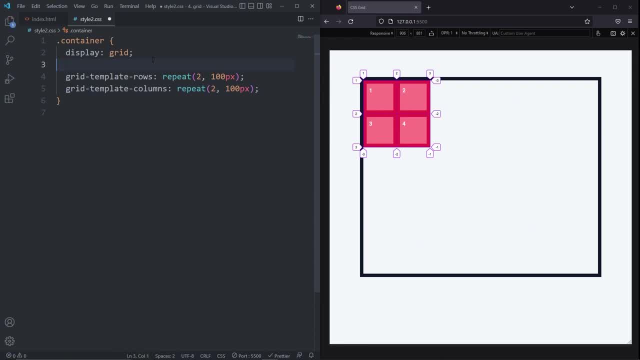 I'll set up a standard grid. The gridTemplateRows can have a repeat of 4- 100 pixels and the gridTemplateColumns can have a repeat of 4, and a min-max of 100 pixels and 1fr If I resize it. 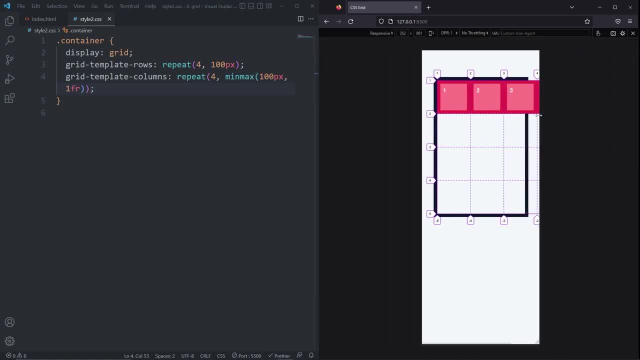 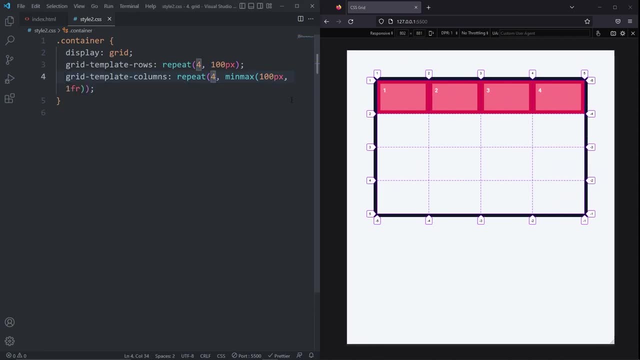 it'll eventually break. To fix this, normally I would add a media query and change things based off the viewport width, but instead all I can do is in my gridTemplateColumns, instead of repeating 4 times, I can replace 4 with the autoFit keyword.